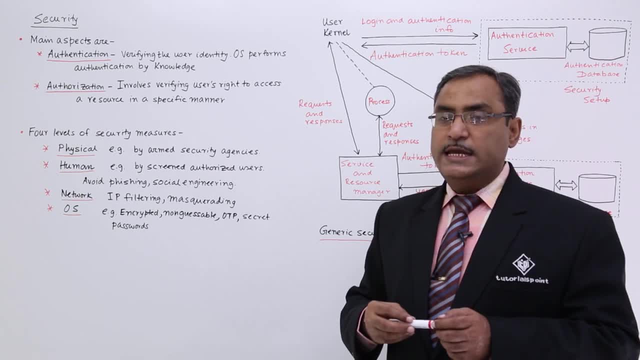 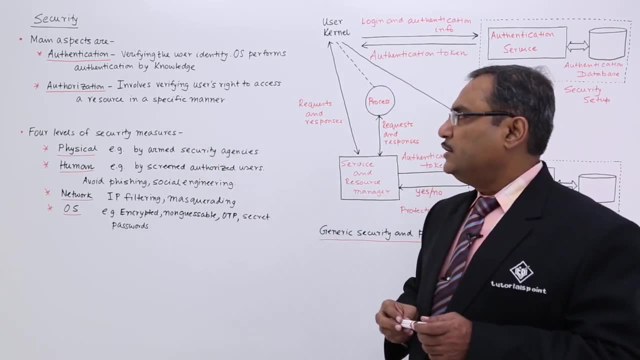 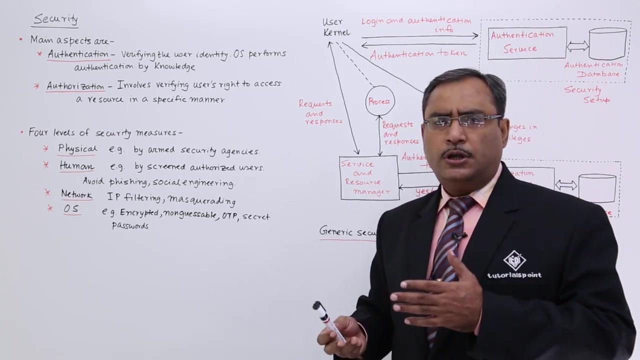 he or she can access and what are the operations he or she can carry out on those resources. so authorization involves verifying users right to access a resource in a specific manner. that means whether he or she can perform the read operation or write operation or update operation, what it can do, what it should not. 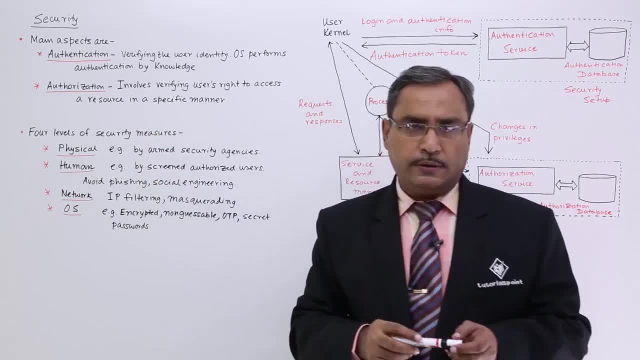 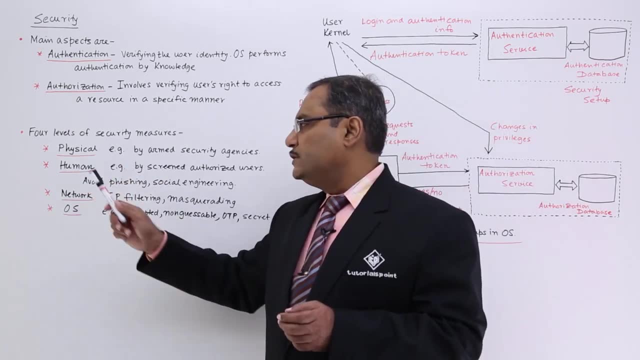 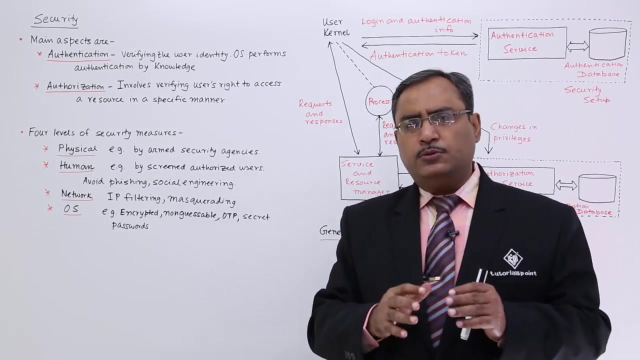 do so. that will be depicted in the authorization aspect and there are four levels of security measures. one is your physical, next one is human network and then os. so in case of physical means, you are giving a physical security to the system. you might be having some armed forces and they are giving that security to the system. 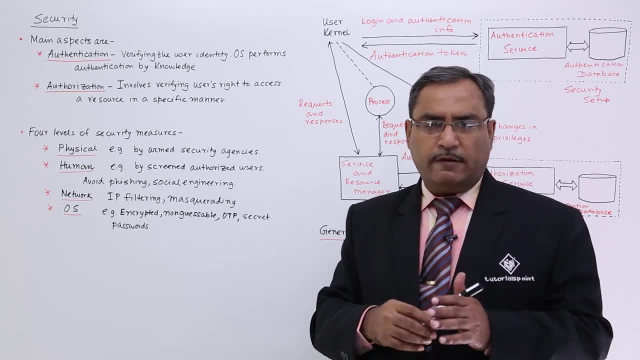 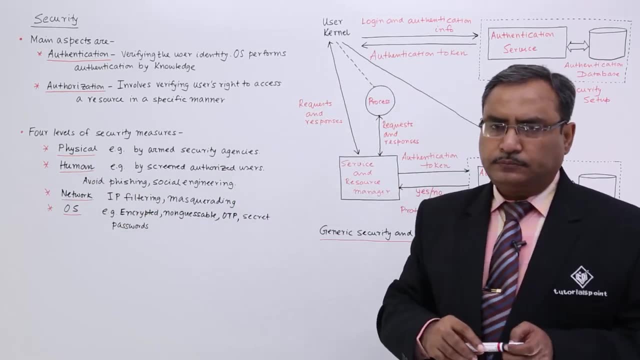 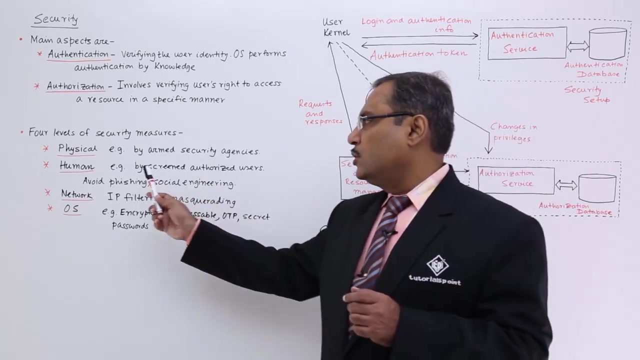 so that means whatever you are doing, you are just making that one physically available, so by the armed security agencies or some other means. in case of human security, that means each and every user should be screened. that means what he is doing or what is not doing. so that sort of level of security should be there. so avoid phishing social engineering. 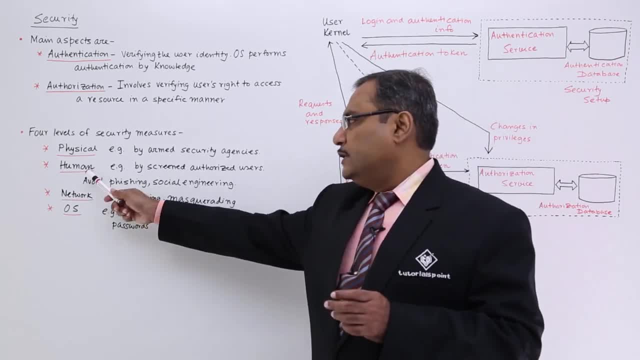 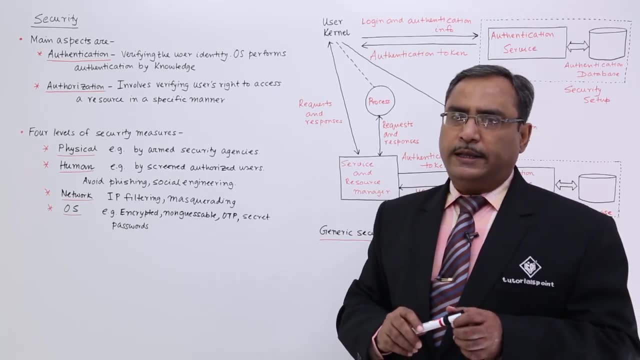 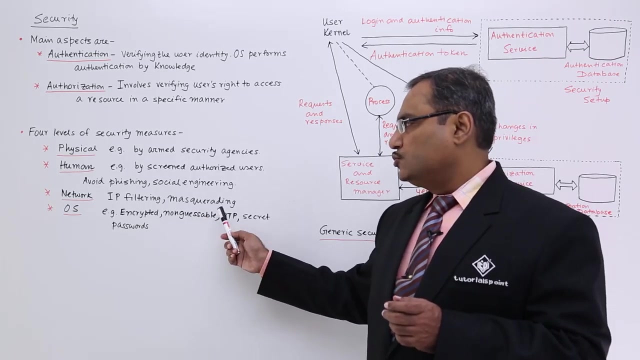 so they may breach the contact. so that is why this human security is very much required. then we are having this network security. so ip filtering, which ip packets can be transferred, which ip packet should be filtered, should be blocked, masquerading. so these are the, these are the methods with the help of which we can ensure network security. that is another. 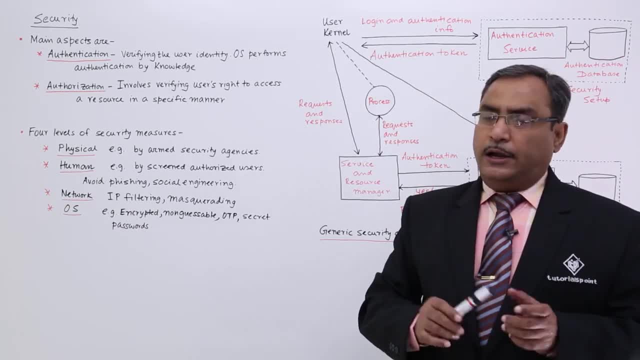 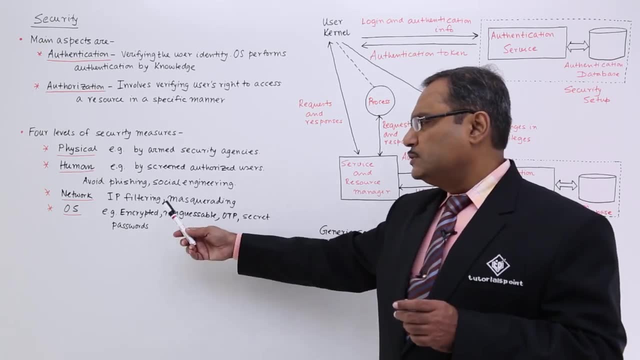 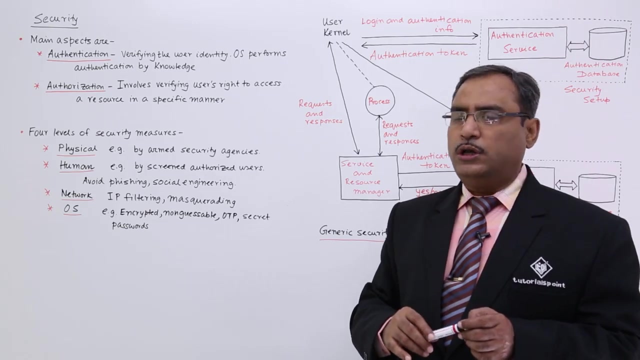 kind of security might be the os. that means i know that we can. in case of os, we can use s. it will have a knowledge to identify the users and it might be through some encrypted passwords. the password should be non-guessable. it might be one-time password, otp it might. 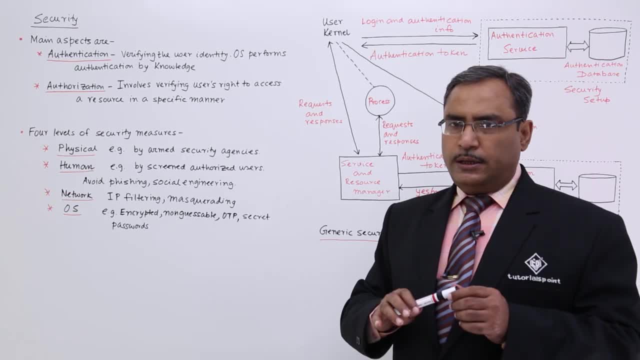 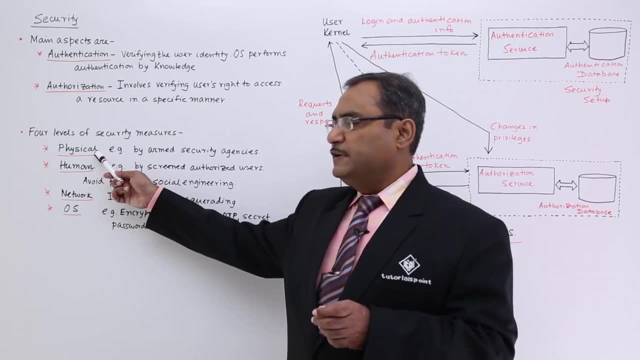 be should be very secret password, and in this way the os security can also be ensured. so we are having four levels of security. one is a physical, next one is human network and os. in this particular diagram i have computerias- the physical, next one is human network and with this particular diagram i have